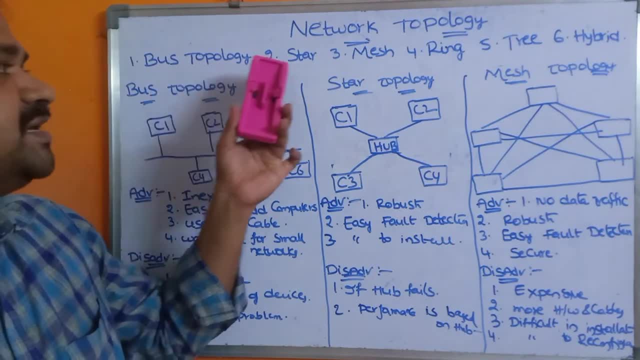 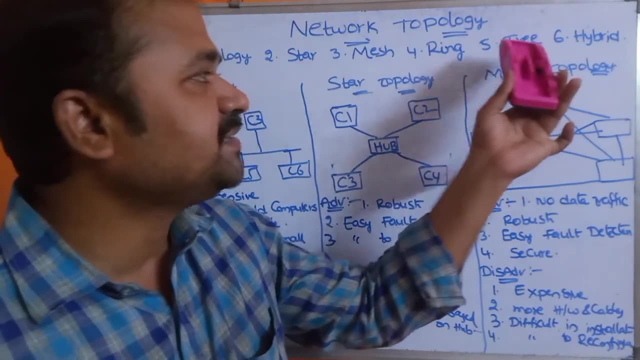 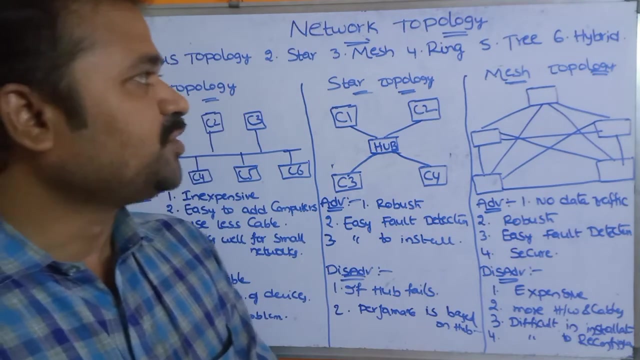 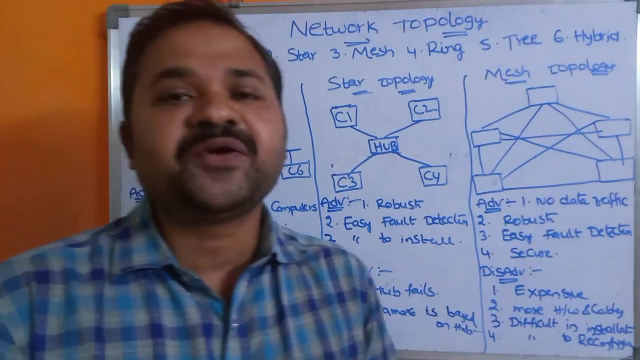 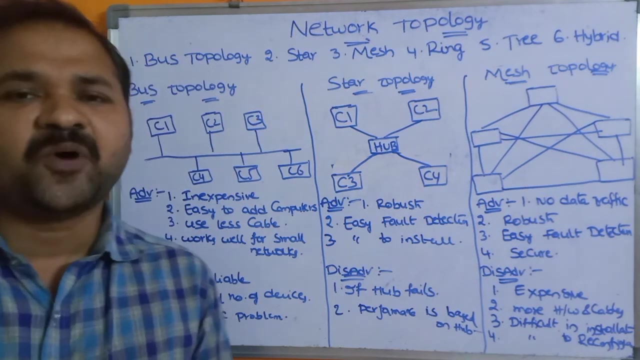 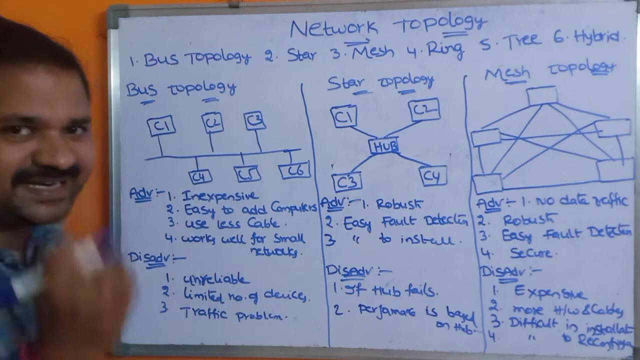 The first topology is bus topology, Second one is star topology, Third one is mesh topology, Fourth, one ring topology, Fifth, one tree topology And the last one is hybrid topology. So here each topology specifies how we are connecting the computers. Let's see the first topology, that is, bus topology. In a bus topology we can have a single cable, So to the cable all the computers are connected. 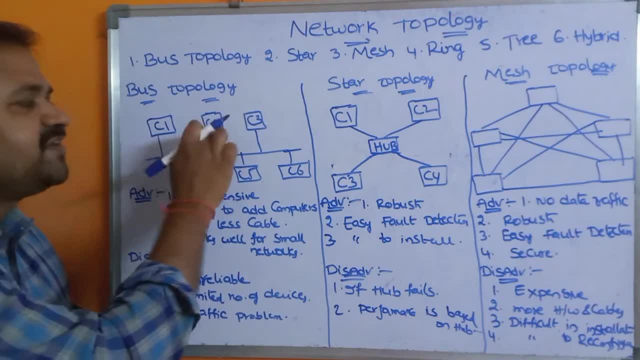 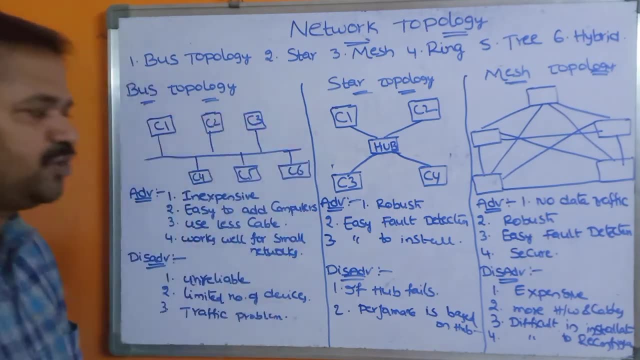 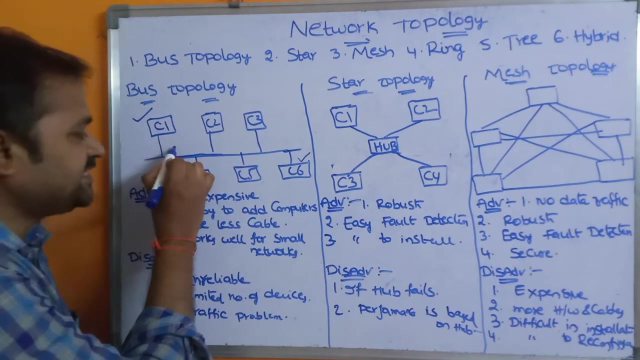 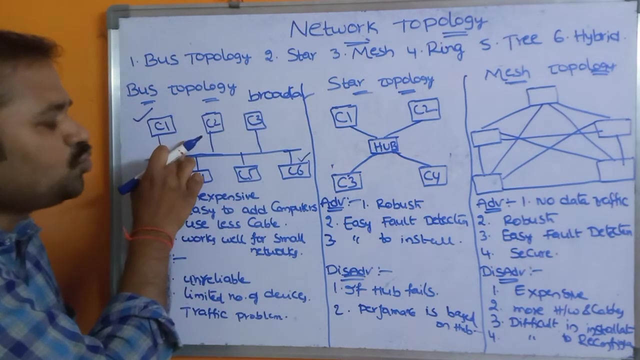 Here we have six computers: C1,, C2, C3,, C4, C6. All the computers are connected. All the computers are connected together with the help of this cable. Okay, Let us assume that C1 wants to send a message to C6. Then it sends the message to C6 with the help of this cable. It broadcasts the message. Okay, It broadcasts the message. So broadcasting means that message will be transmitted to all the computers which are connected in that network. Okay, So C2 has that message. 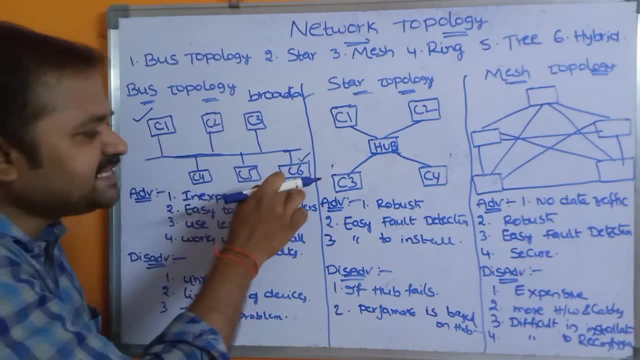 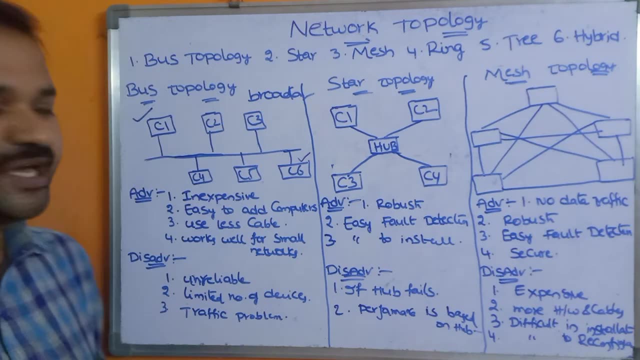 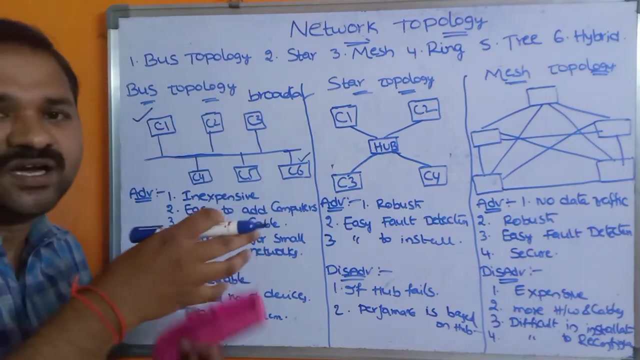 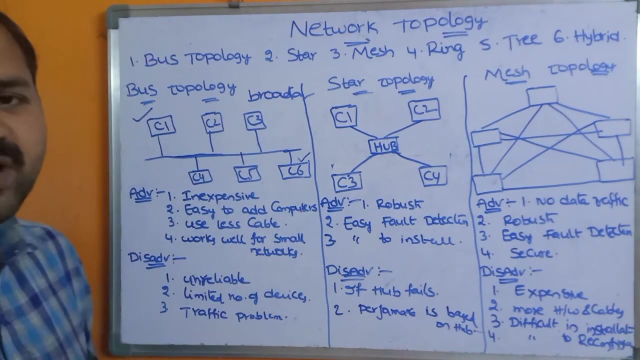 C3 has that message, C4,, C5, C6 has the message Here. the advantage here is the message contains destination address. Okay, Here that message contains C6 address. So now C6 will reach that address. So, based upon the address, C6 will reach the message. So the remaining computers won't reach the message. Okay, Why? Because that destination address won't match with these computers: C1,, C2,, C3. 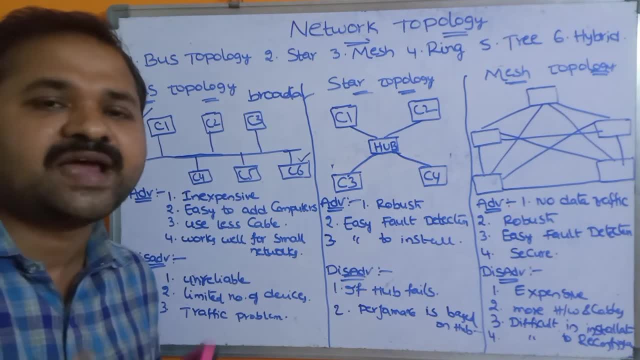 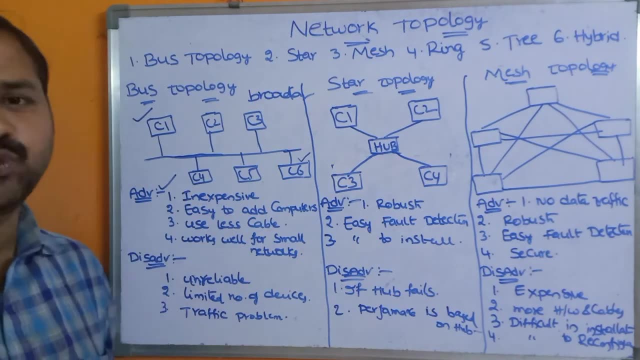 2, c, 3 c, 4, c, 5. okay, now let us see the advantages and disadvantages of this approach. the first advantage is: it is very, very inexpensive. why? because we require only one cable. so to the cable all the computers are to be interconnected. the second advantage is easy to yard additional. 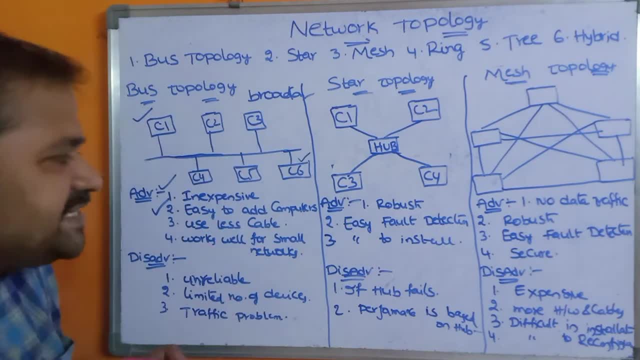 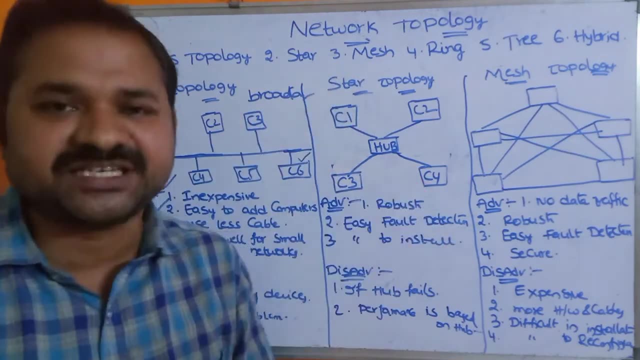 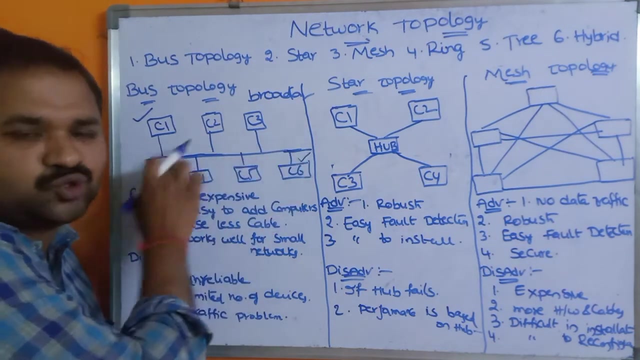 computers. let us assume that i want to insert, i want to add five more computers. so simply to the cable, all those five computers will be attached. and the third advantage is use less cable. okay, here only one cable is needed. so to the cable. all the computers are to be connected. the next: 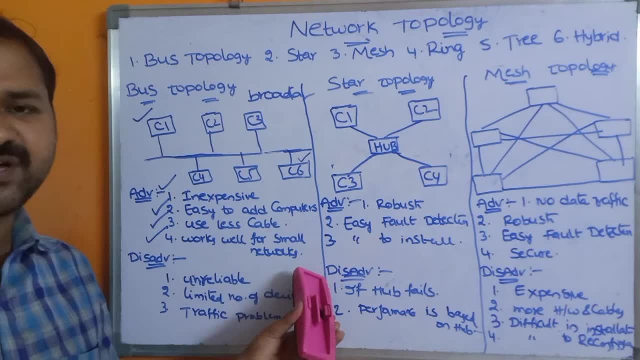 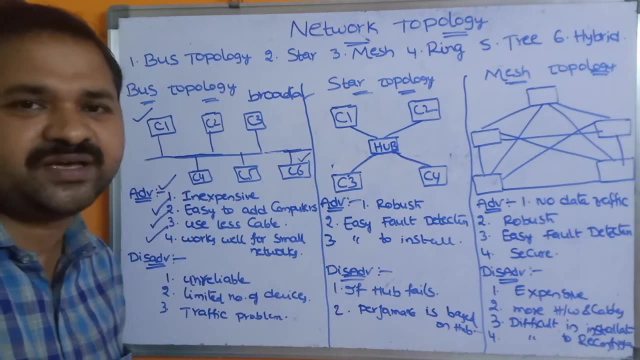 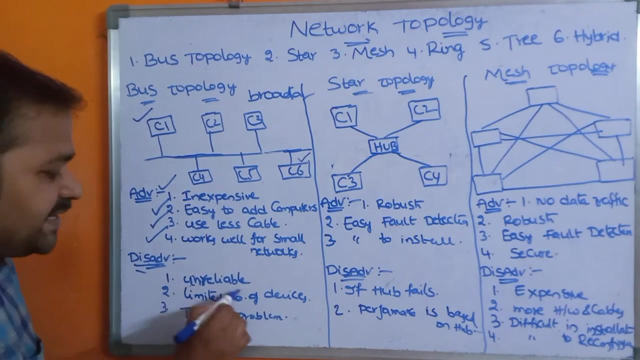 advantage is: works well for small networks- okay. it is more suitable for the smaller networks. let. it supports 100 computers. okay. beyond 100 computers, it cannot support that one. okay. let's see the drawbacks here. first drawback is unreliable. unreliable why? because if this cable fails, then the entire. 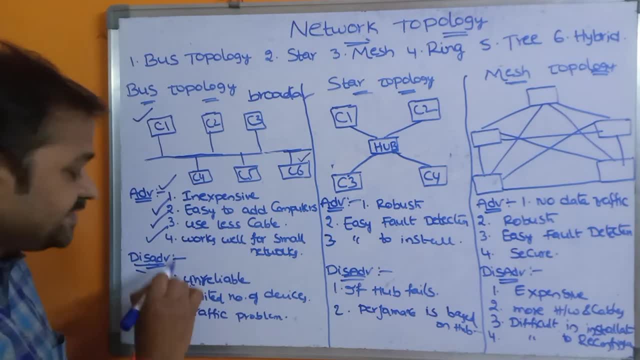 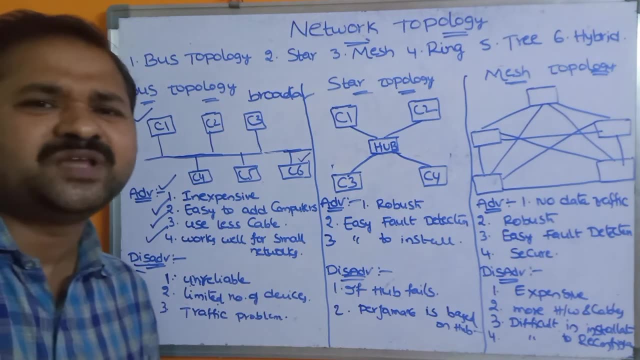 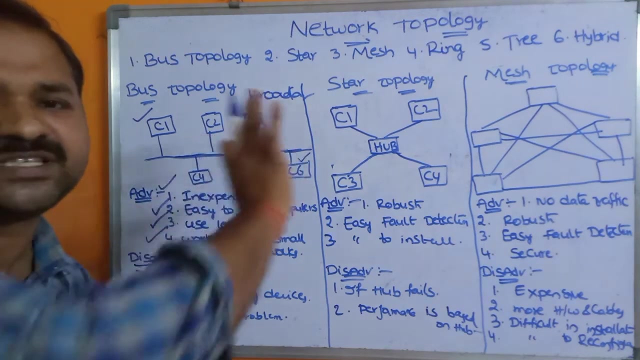 network will fail, okay, so that's why we can say that this is unreliable approach. and the second drawback is limited number of devices. let us assume that we can attach only 100 computers to the cable, okay, so beyond that it is not possible to attach the computers. and the third problem is: 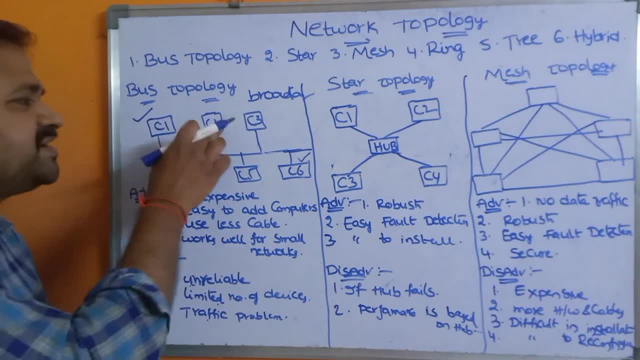 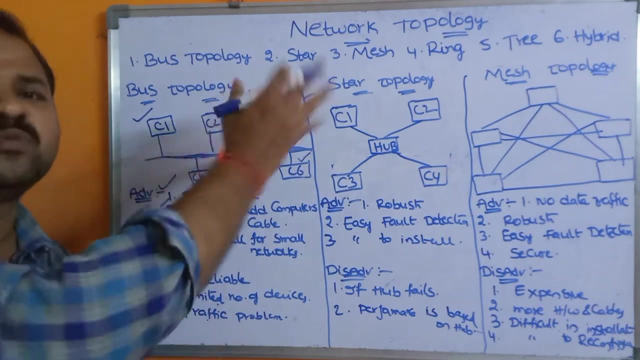 traffic problem. there is a possibility that if we attach C1, C2, C3 may transmit the message simultaneously to the C4, C5, C6. but here what we are using, we are using single cable, so through this cable only that message will be transmitted. so there is too much of traffic here. why? because three messages are. 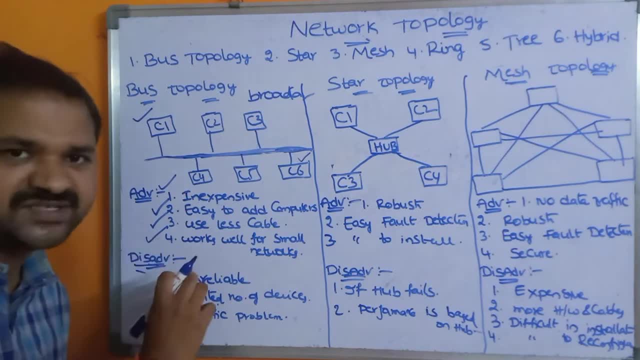 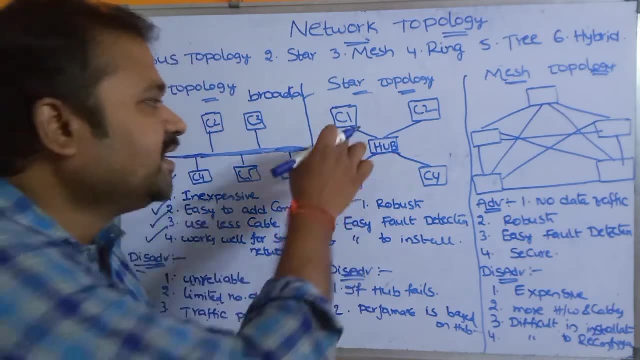 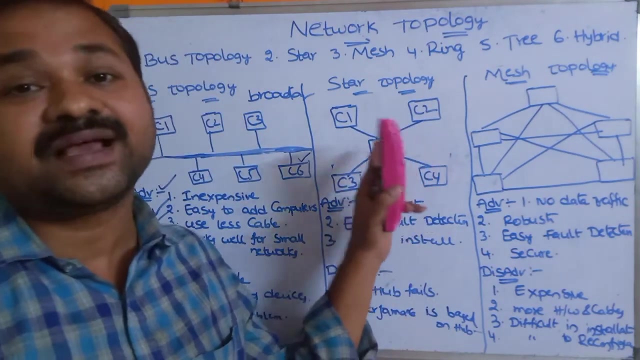 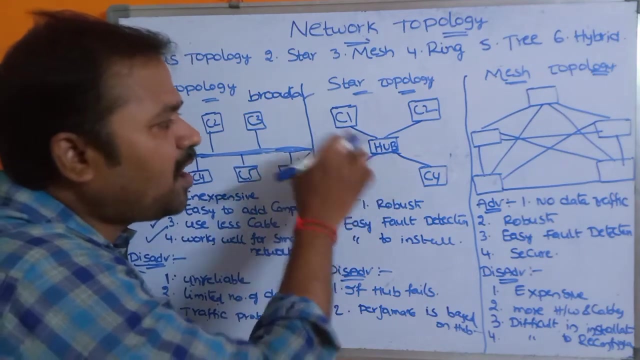 transmitting now with the help of this cable. so these are the drawbacks of this approach. okay, now let us see the second approach, that is starto policy. in starto policy have multiple computers. all those computers are connected to a central point, a central device such as hub. so here we have a hub. so to the computer, to the hub, all the computers are. 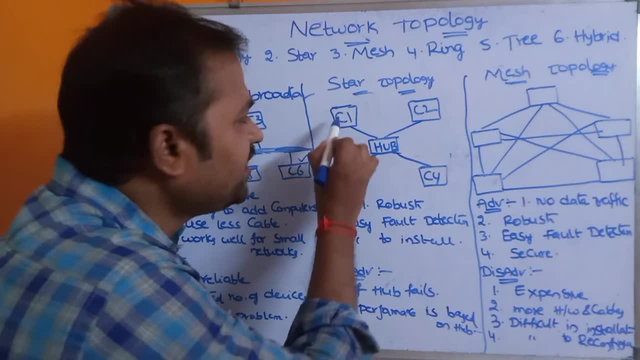 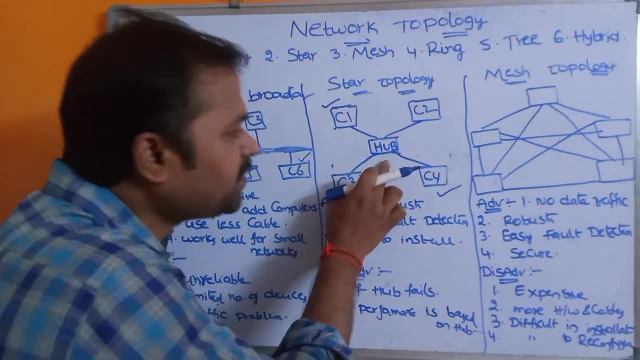 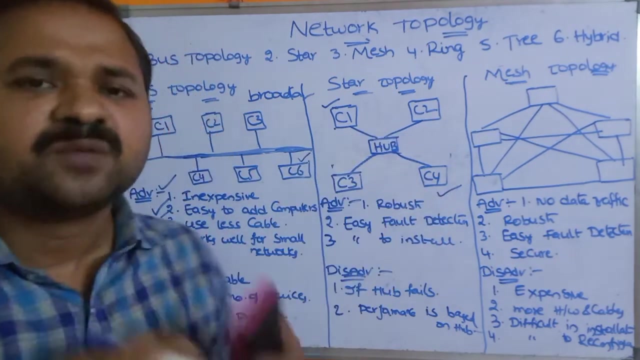 attached. okay, let us assume that c1. c1 wants to send a message to c4. now what will happen is c1 sends the message to hub. now that message is available in the hub, so from the hub that message will be transmitted to c4 based on the destination address. okay, so directly. the transmission won't. 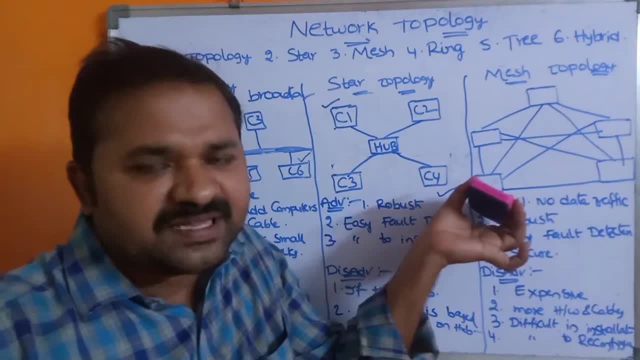 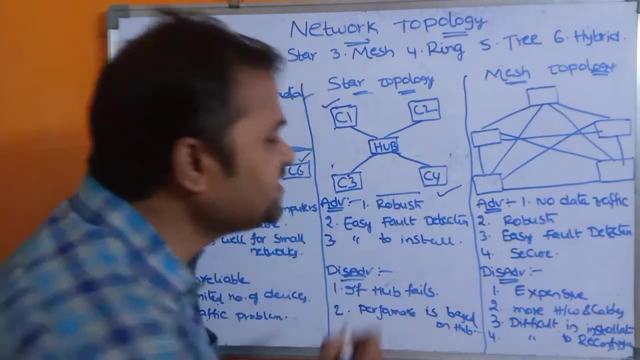 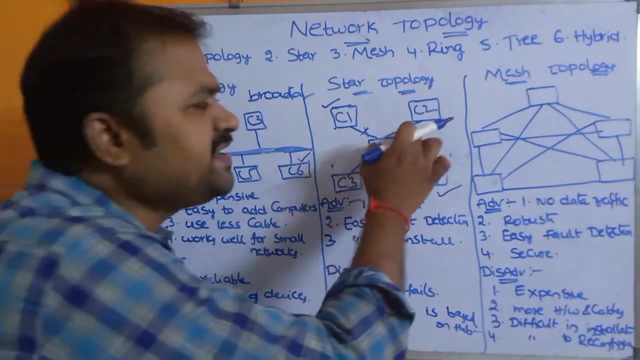 done here. so hub stores the message from the hub. that message will be delivered to the corresponding destination. now let us see the advantages and disadvantages. the first advantage is robust. robust means it is very, very strong. if one link fails- let us assume that this link fails- then the remaining links won't fail. we can use the network, there is no problem. and the second: 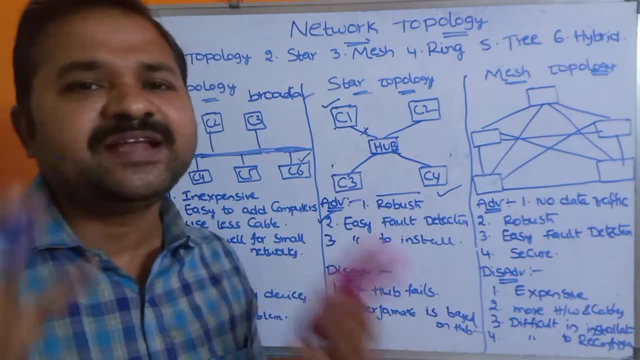 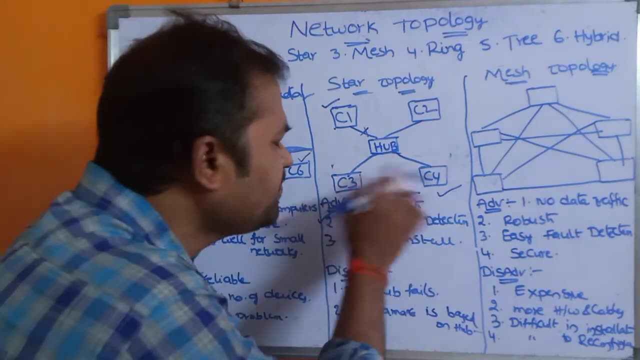 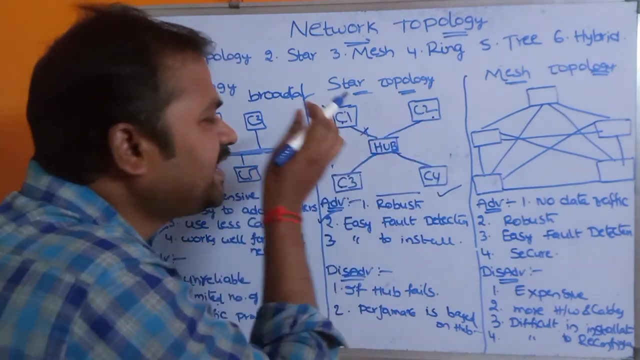 advantage is easy fault detection. that means if there is a problem with a specific system, then we can detect that system very, very easily. why? because here all the computers are nothing but some neighboring computers. only if there is a problem with c1, then c2 or c3 can detect that problem very, very easily. 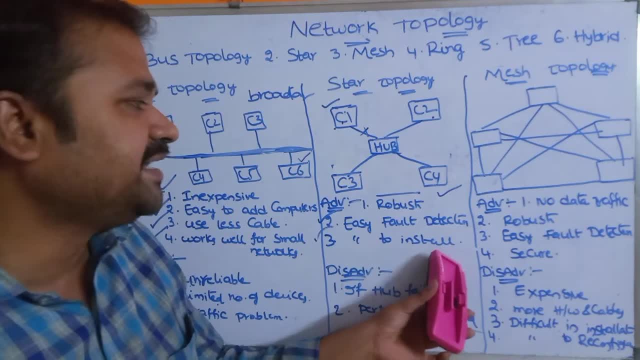 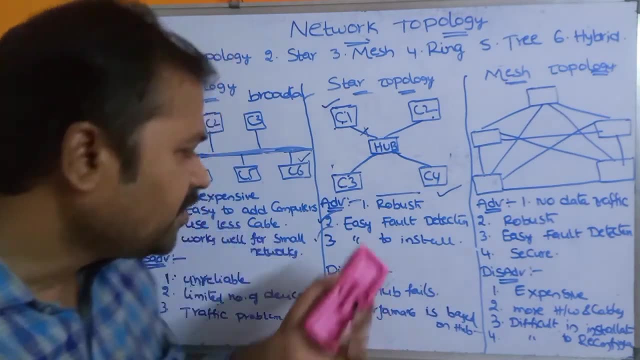 and the third advantage is easy to install. easy to install why? because here we have only one hub. so to the hub all the computers are to be connected. okay, now let us see the drawbacks here. if the hub fails, then the entire network will fail here. okay, here the hub is. 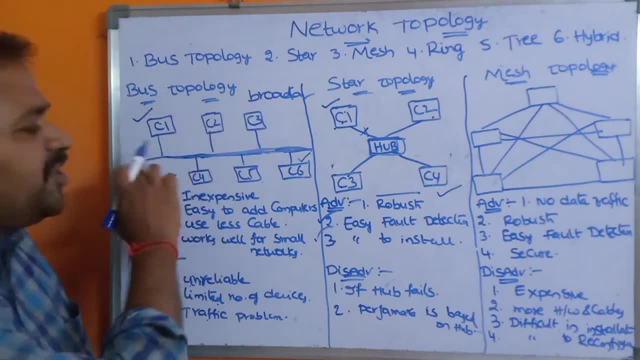 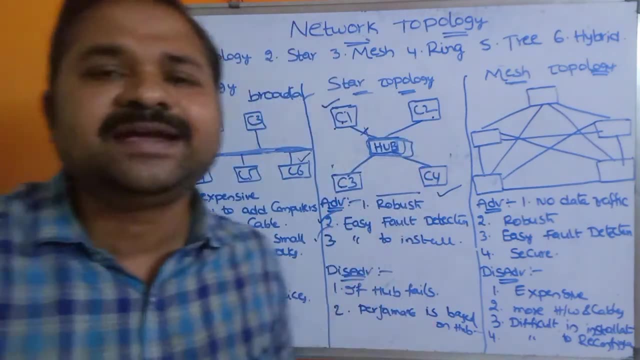 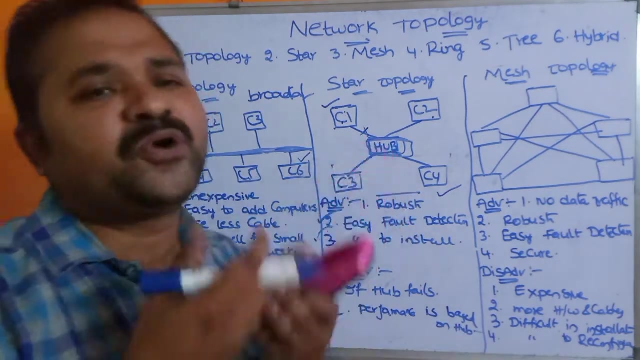 very, very important. just like in bus flow policy, this cable is very, very important. so likewise here the hub is very, very important. if hub fails, then the entire network will be collapsing. and let's see the second problem here. performance is based on the hub. here, if hub produces higher, 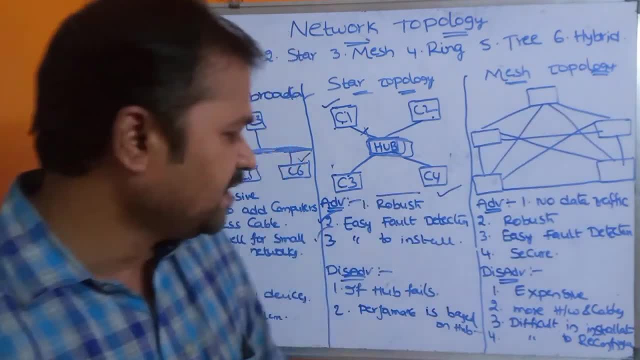 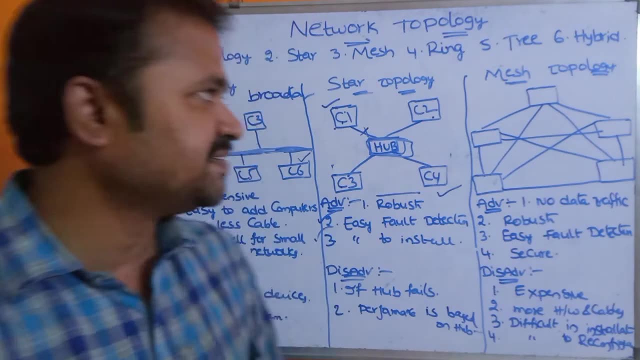 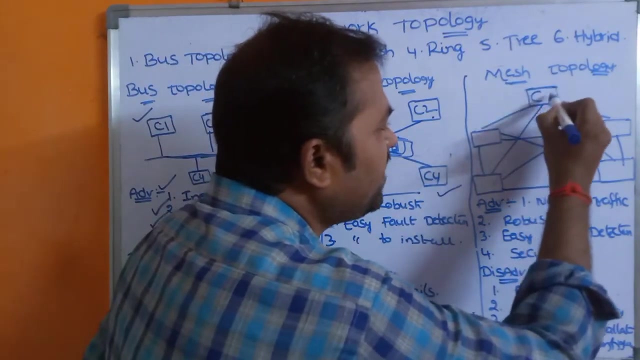 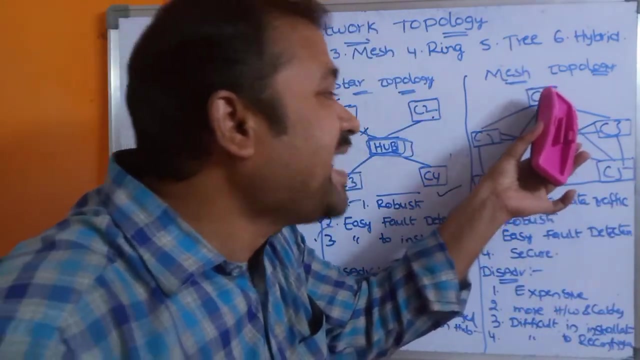 performance, then the network will produce a higher performance. okay, if hub produces lesser performance, then obviously the remaining computers and the network will produce less performance. now let us see about the next one, that is, mesh topology. in mesh topology what will happen is here we have several computers like this: c1, c2, c3, c4, c5- so from each computer we have links to remaining all the. 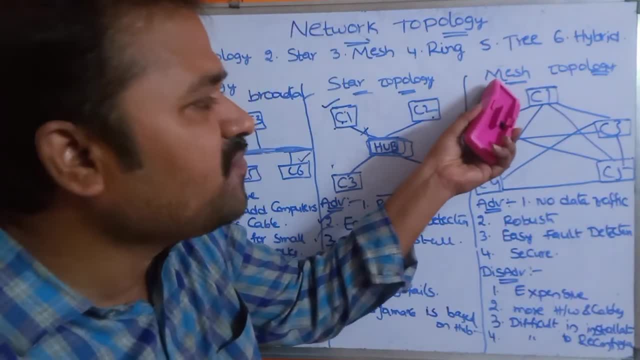 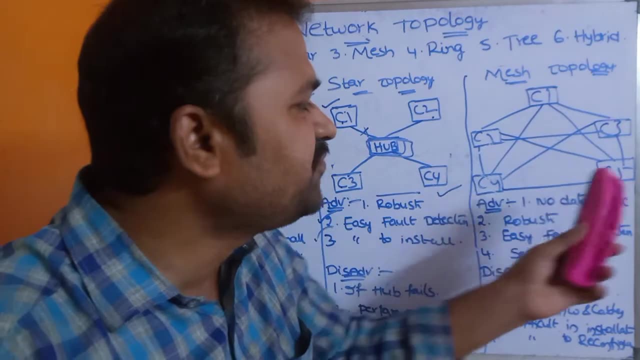 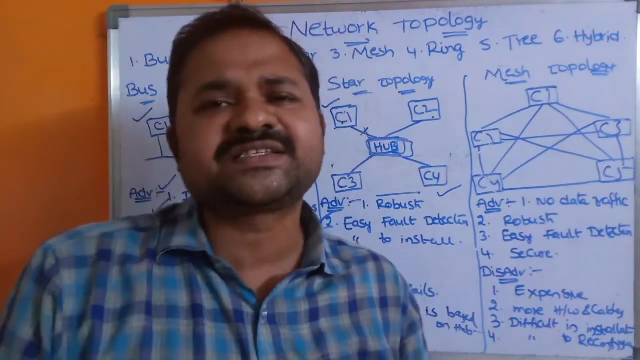 computers in the network. okay, so from c1 we have links to c2, c3, c4, c5. next, from c2 we have links to c� 1, c3, c4, c5. so this is about mesh topology. okay, so from one device, two, remaining all other devices. 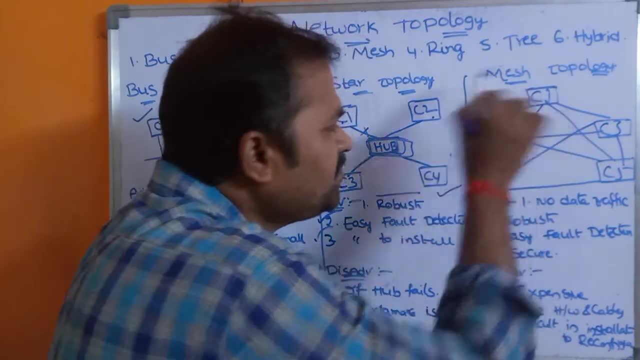 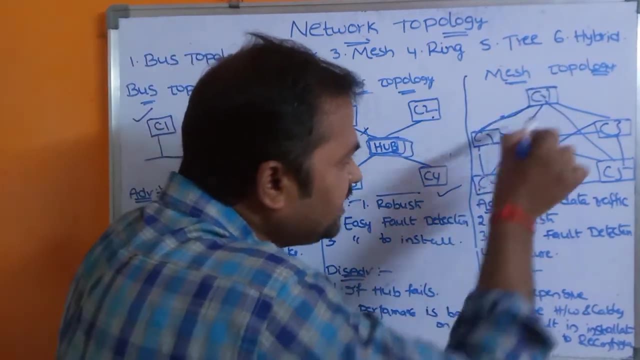 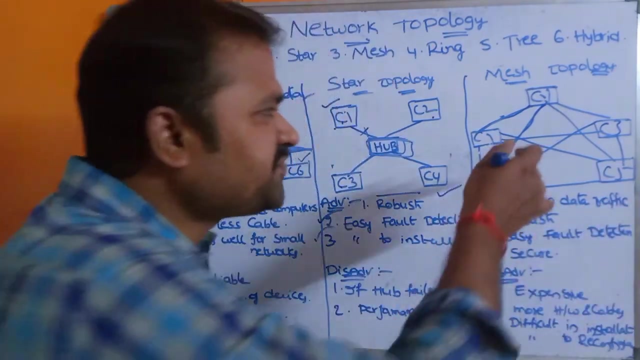 we should have the corrections. let us assume that if c1 wants to send message to c2, then for that, if uses this link, only okay. let us assume that c1 wants to send message to c4, then if uses this link, only okay. let us see the advantages here. there is no data traffic here. 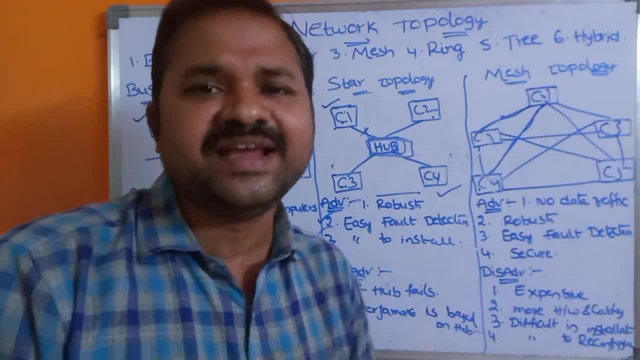 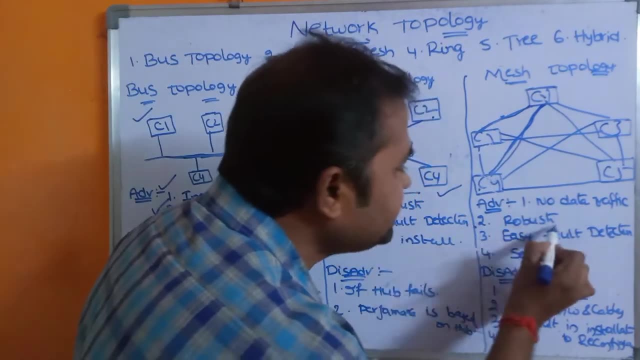 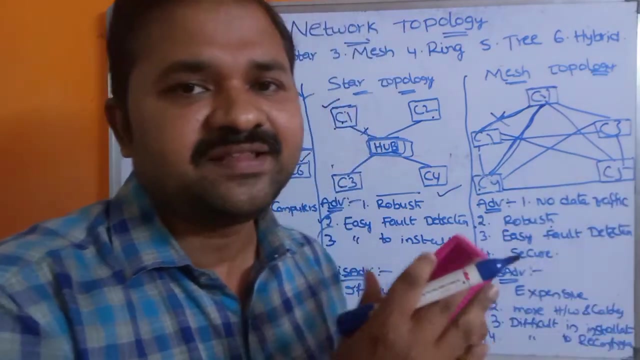 why? because from each device, other devices, we have the links. so with the help of that link, data will be transmitted. so there is no traffic, okay. and the next advantage is it is very, very robust. it is strong. if one link fails, there is no problem, the remaining links will works and the network. we can work with the network. 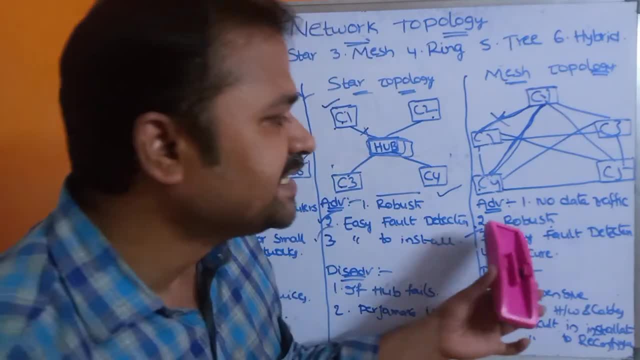 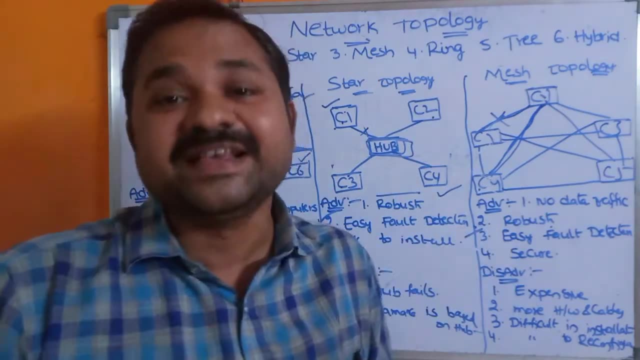 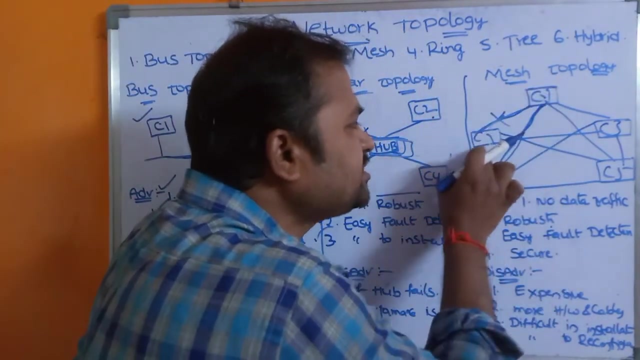 there is no problem for the network. and the third advantage is easy fault detection. here also, if there is any problem with particular system, we can detect that fault very, very easily. okay, and the fourth one is: this approach is very, very secure. why? because c1 can send message to c2. 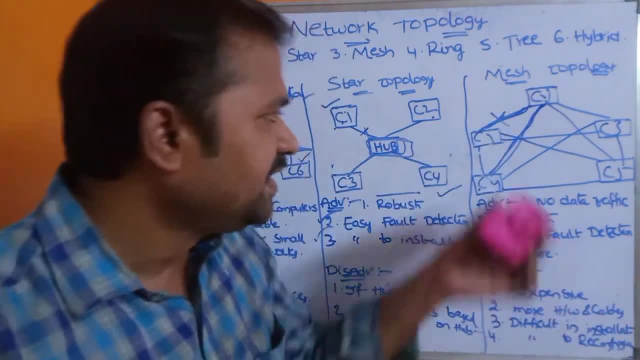 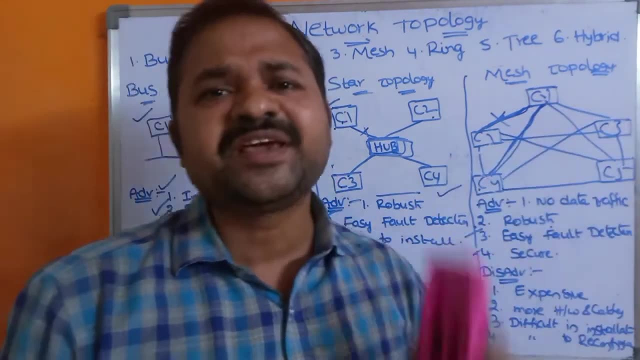 with the help of this link, so nobody can watch our data. okay, directly. with the help of the link, we can share the data. and the problems are: it is very, very expensive approach. why? because too many cables are needed. okay, so here the formula here is: if there are n computers, then from that computer. 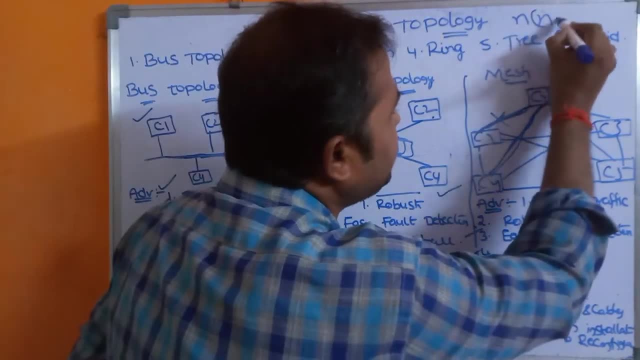 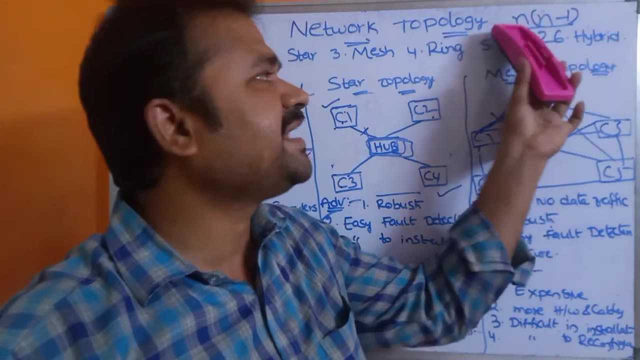 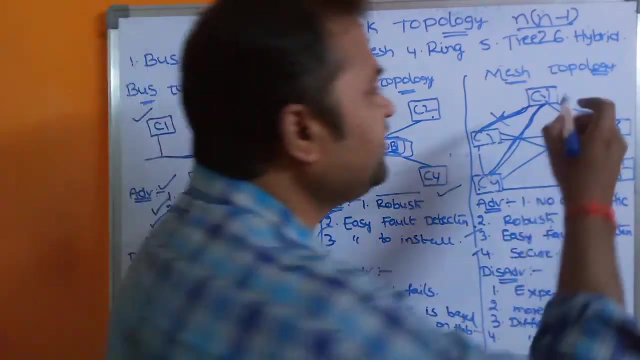 to remaining all computers. okay, we need to establish the connections. so here the formula is any to n minus 1 by 2. if there are n computers, then we require n into n minus 1 by 2. connections: 2 links here. what is n value? 1, 2, 3, 4, 5, so 5 into 5 minus 1 means 4, so 5 into 4 by 2 means. 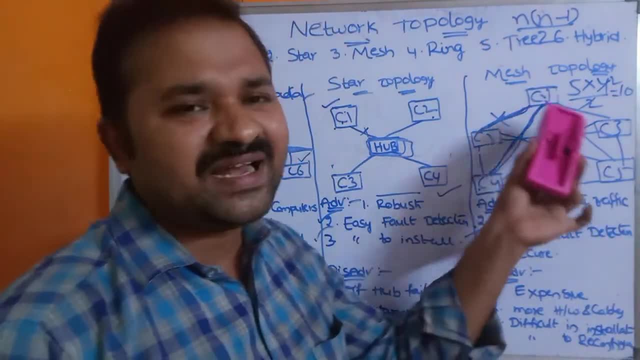 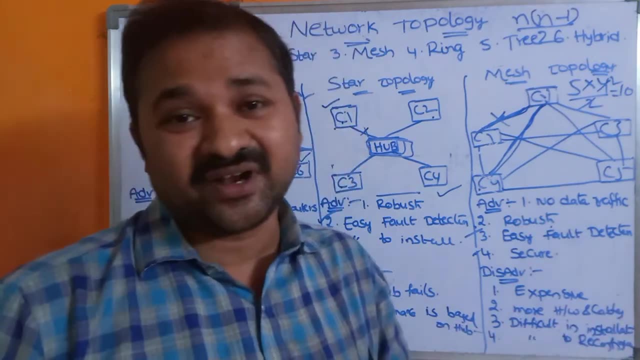 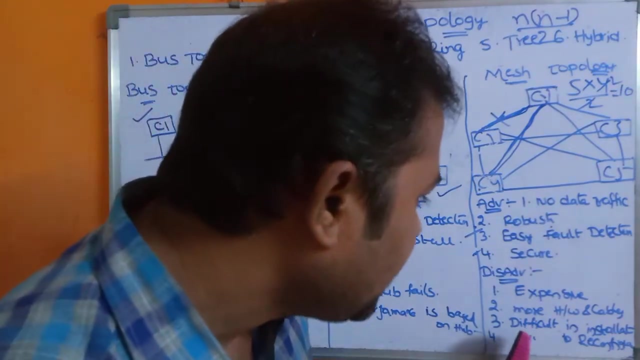 10, so we require 10 links here. okay, we require totally 10 links here. so too many cables are needed, so it is very, very expensive approach, as well as if required more hardware also why? because many number of cables are required, so more hardware will be required. so it is very, very costly approach and difficult in installation. why? because from 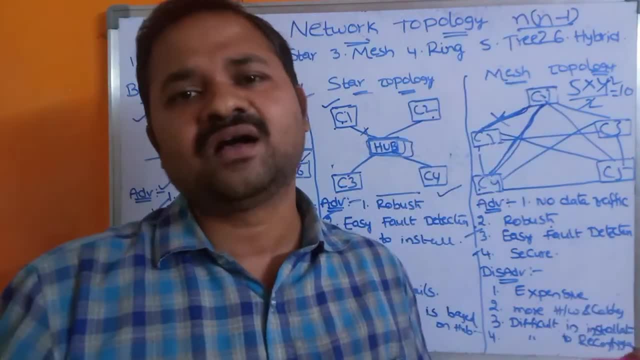 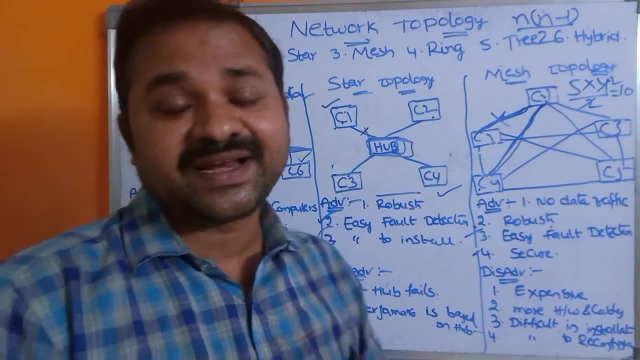 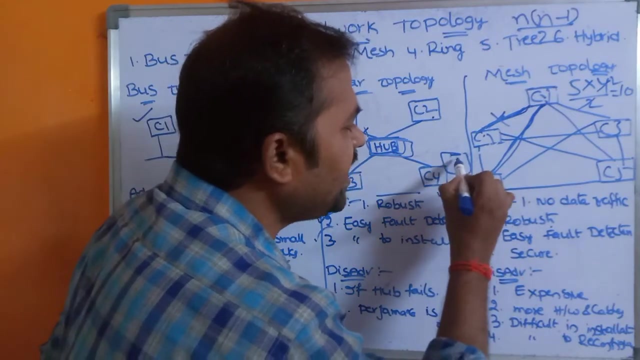 each computer to remaining all the computers we have to make the links. so it is very, very difficult to implement this approach, also difficult to reconfigure. so reconfigure means let us assume that we want to add some additional computer. so in between c2 and c4 i want to add 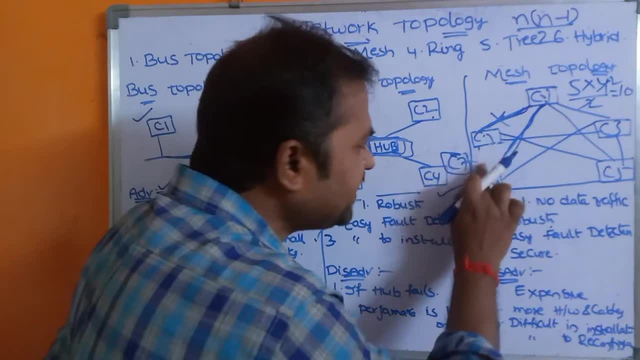 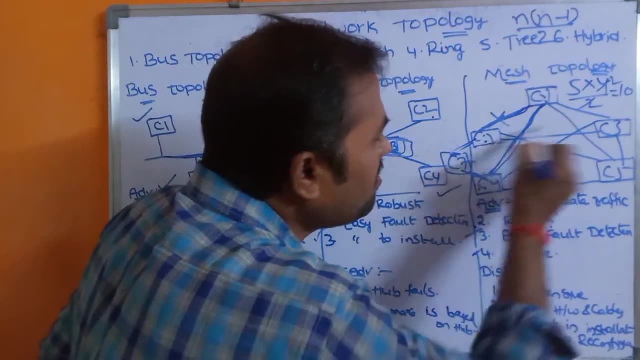 some c7 system, then what we have to do? we have to remove this connection. we have to remove this connection and we have to make the connection like this: okay, next, from this computer to remaining all the computers. we have to make the connections from this computer to remaining all. 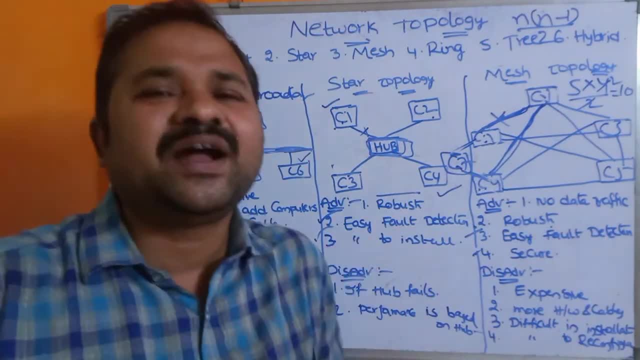 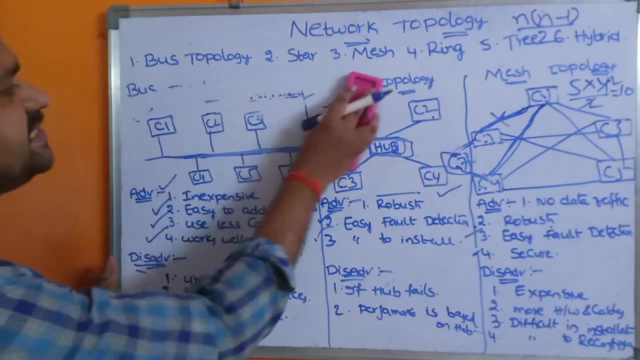 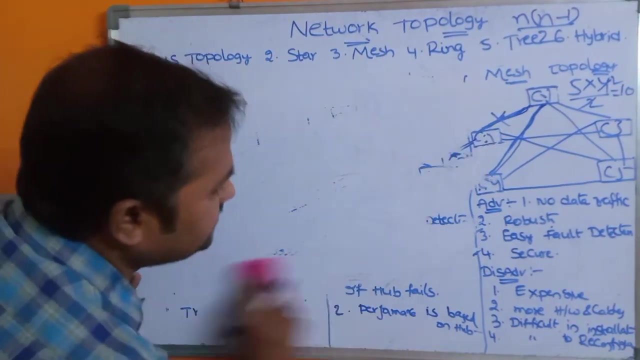 the computers. we have to make the connections. so if you want to add an additional computer, then it is very, very expensive. approach, okay. and the fourth one is a ring topology. so let us see about ring topology now. a ring topology, so ring topology means it follows some links, some ring architecture. 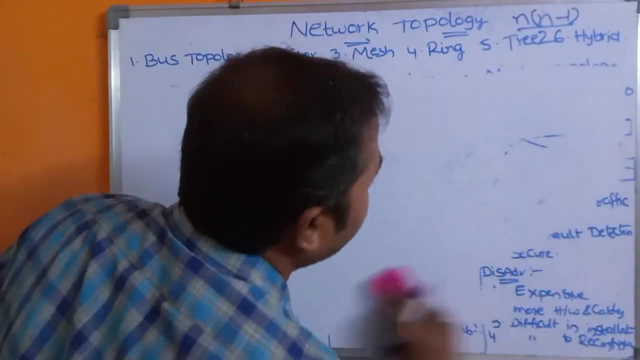 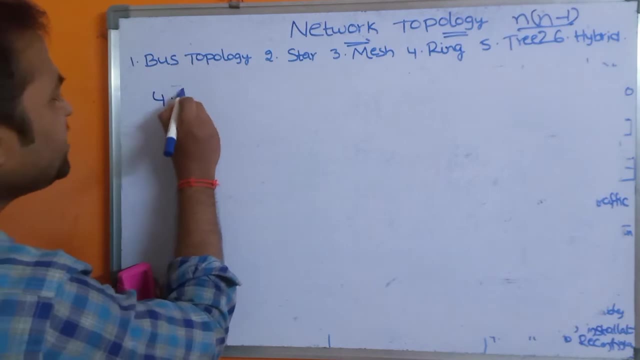 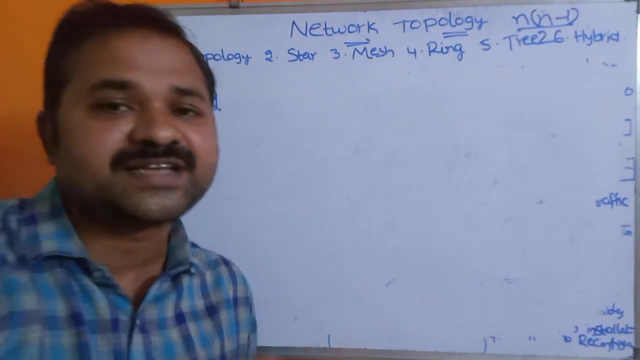 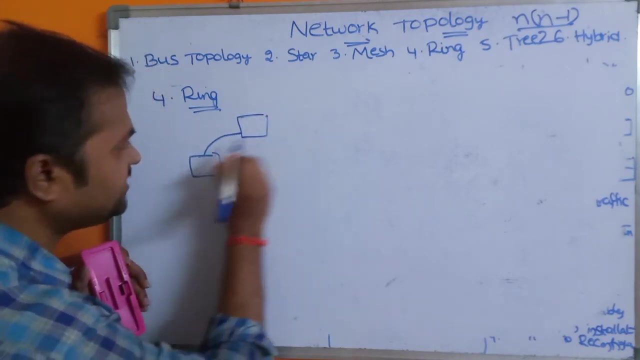 ring architecture. so next we have three topology: hybrid topology. let us see about those three now. so the next one is ring topology. in ring topology what we have is each computer will be connected to its adjacent computers, it's neighboring computers. so like we have a computer like this, then this computer will be connected to its neighboring computers like that. okay. 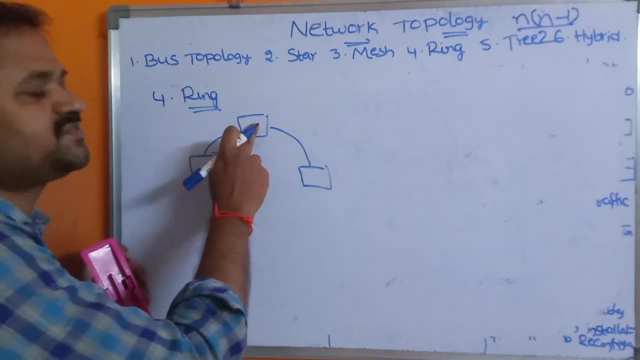 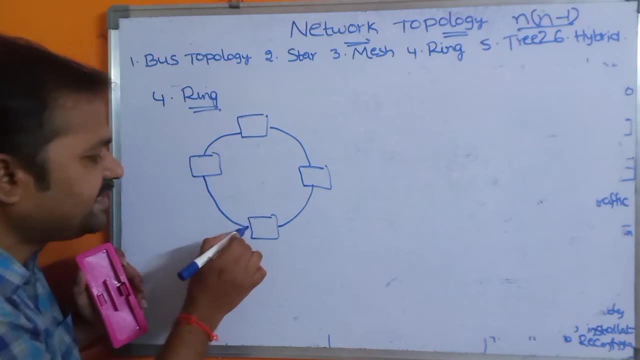 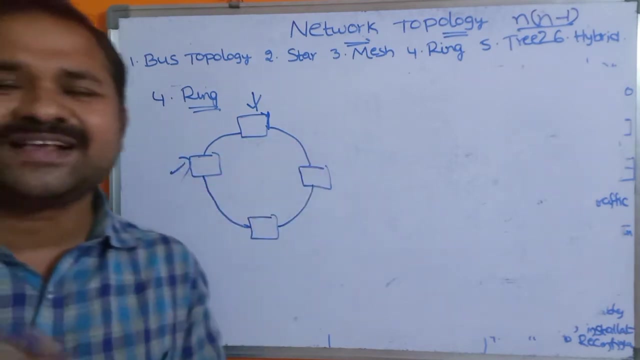 and this computer is connected to its neighboring computers. so this is one neighbor and this is the second neighbor, and and these computers, these two are connected like this. okay, so let us assume that this computer wants to send message to this computer. here the transmission of the data is unidirectional. unidirectional means. 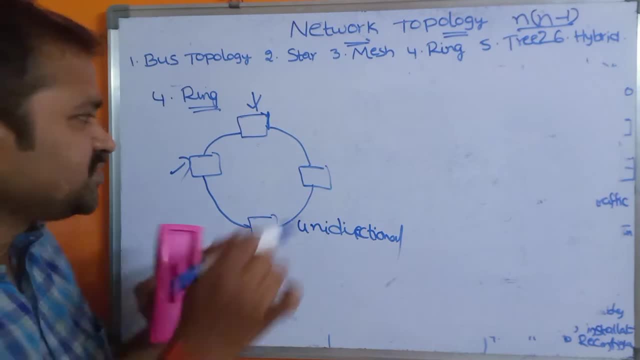 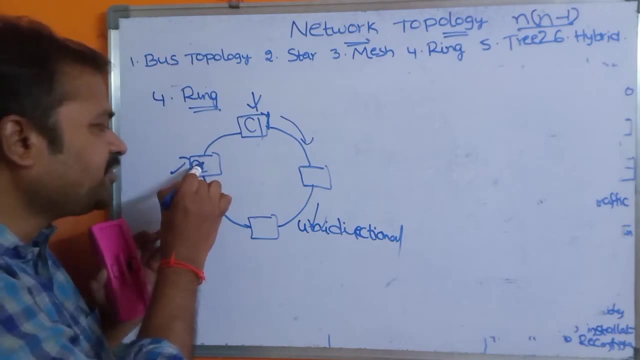 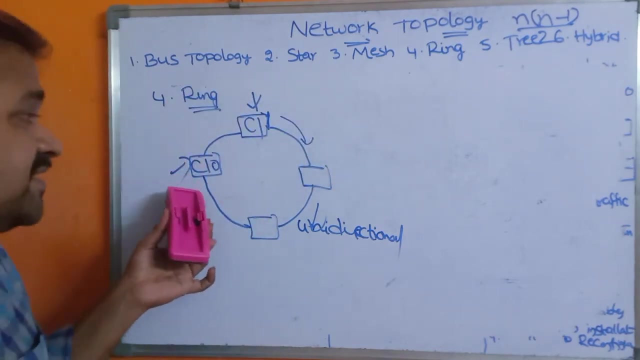 the data will be transmitted in only one site. okay, so the data will be transmitted like this. okay, let us assume that this is first computer. this is last computer. computer number is some 10 if the computer number is 10. so if c1 wants to send message to c10, 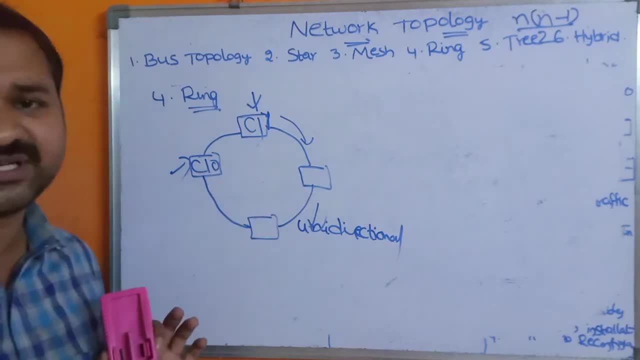 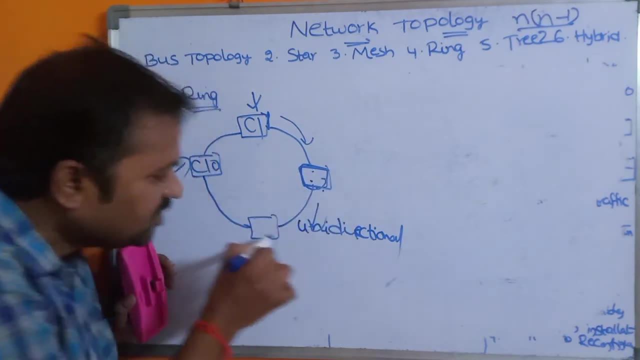 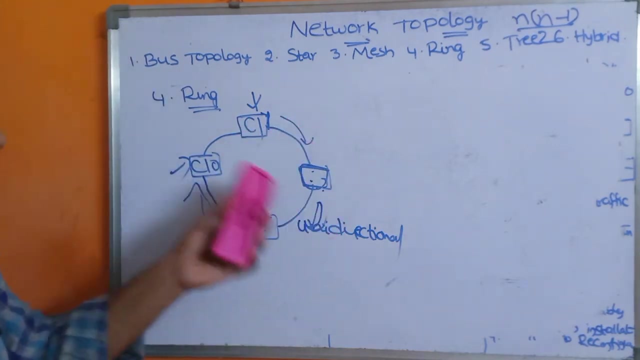 then it has to travel through the remaining nine computers. okay, so first the message will be transmitted to this computer. now that now this computer passes this message to this computer, now this computer passes the message to this computer, so likewise the message will be transmitted from one computer to one computer language. okay, now let us see the advantages. 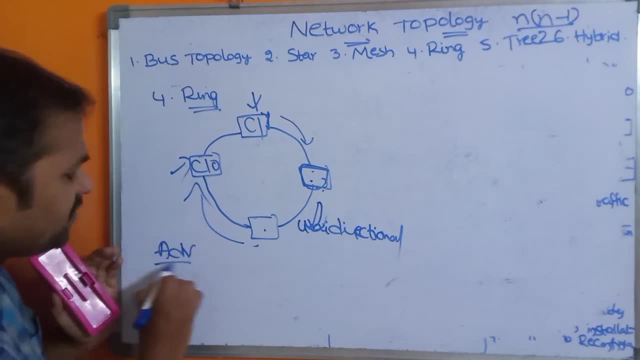 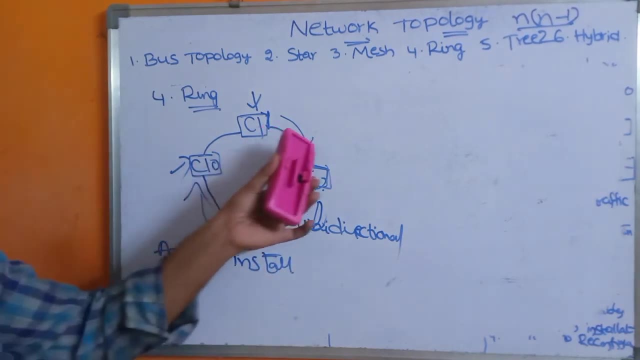 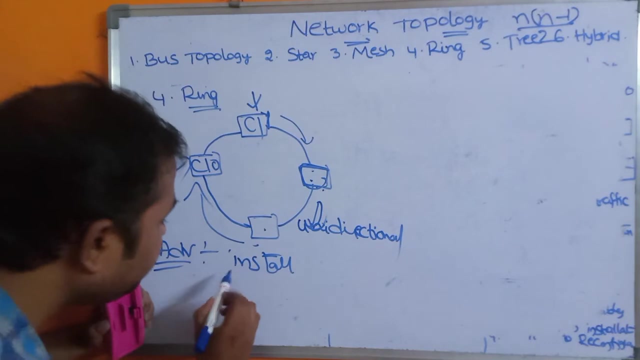 and disadvantages of this approach. the first advantage of this approach is it is very, very easy to install. we can implement this approach very, very easily. why? because we need some tables. so with the help of those tables we can, we can establish the architecture. and the second advantage is it is very, very inexpensive approach. it is very, very. 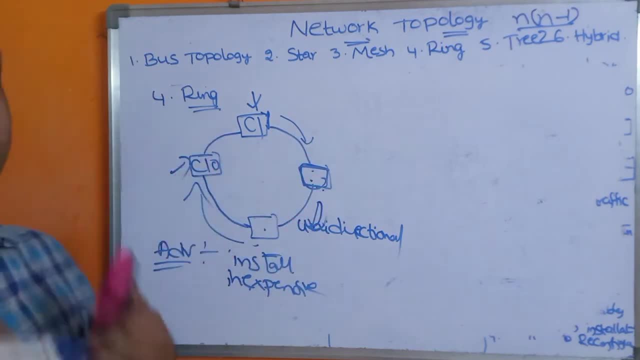 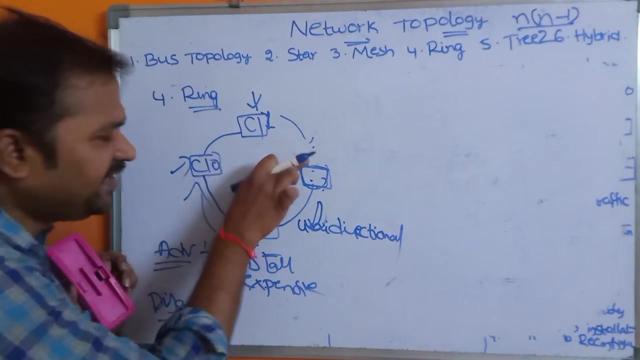 inexpensive approach. why? because less number of tables are needed when compared with mesh architecture, mesh technology, various. the drawback back with this problem is: suppose if one link fails, if one link fails, then the entire network will fail. suppose let us assume that this link fails. if this link fail, then c1 can't send the. 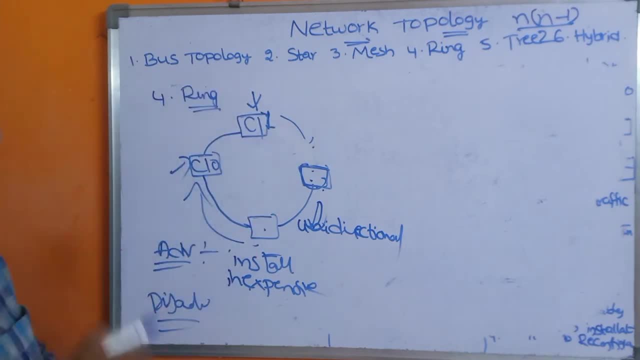 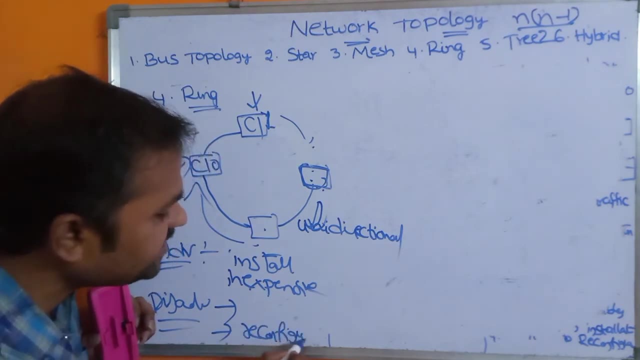 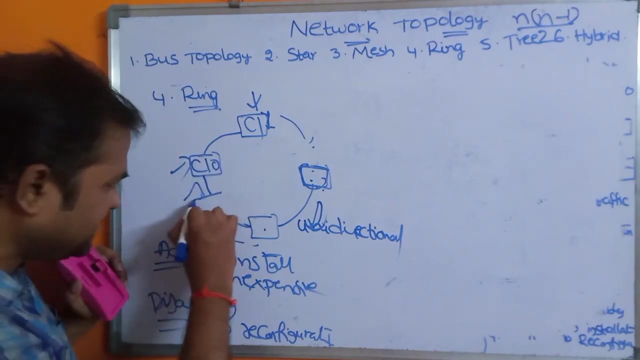 message to the c2, so this message won't be sent to c10. okay, and the next problem here is reconfiguration is very, very difficult. what is reconfiguration? let us assume that i want to insert a new computer into the token tree. let us assume that i want to insert at this position: 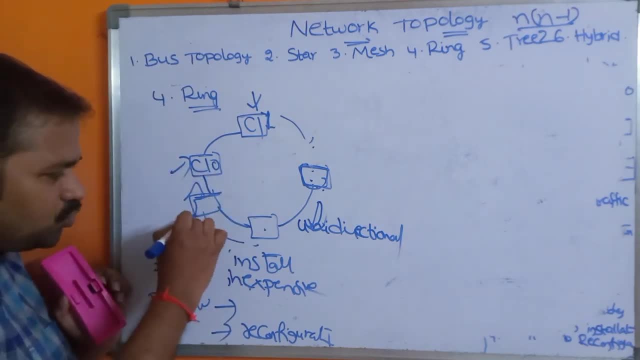 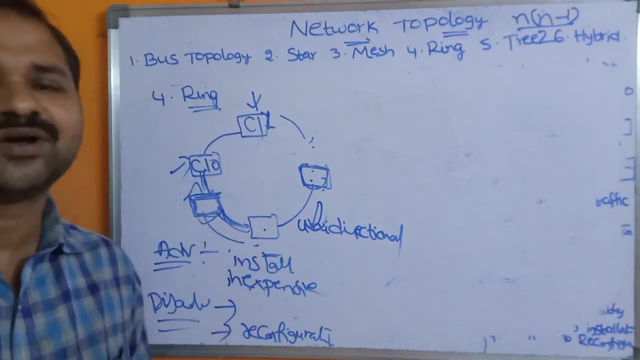 so now we have to remove these two connections and we have to, we have to insert the computer here and we have to make two more connections like this. okay, so reconfiguring is also very, very difficult in this approach. and the next one is tree topology. tree topology- tree topology. 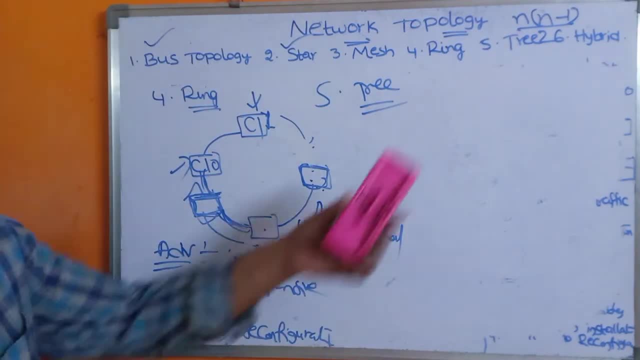 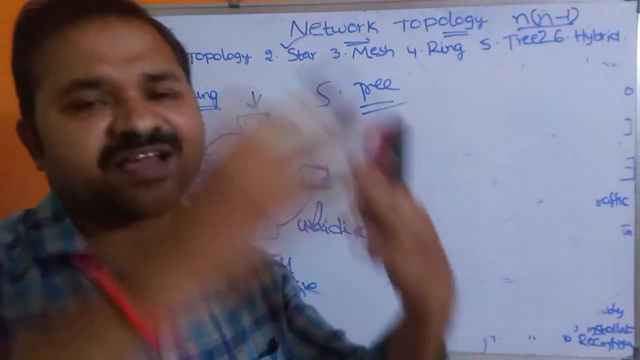 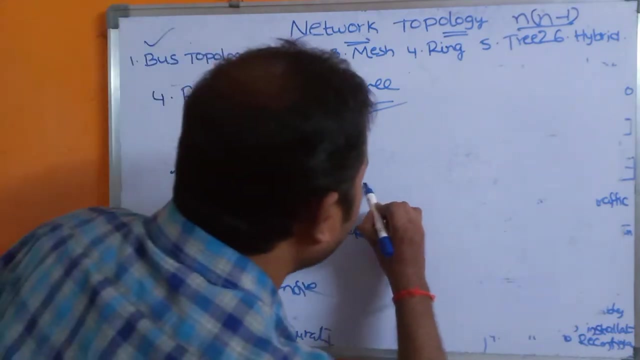 is a combination of bus and star topology. so tree means it is a combination of bus and star-toe policy. So we know what is a tree. Tree means a collection of nodes and it is useful to represent hierarchical information. So here we can have multiple levels. So here we have a cable. 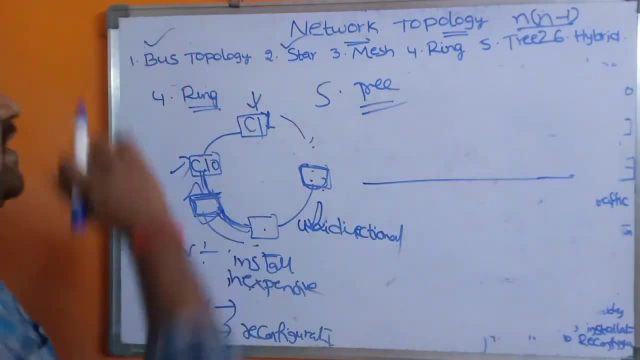 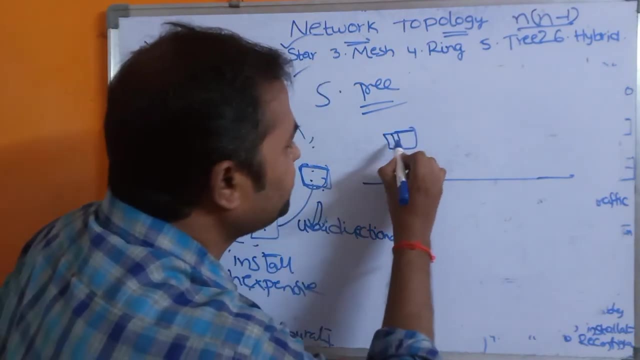 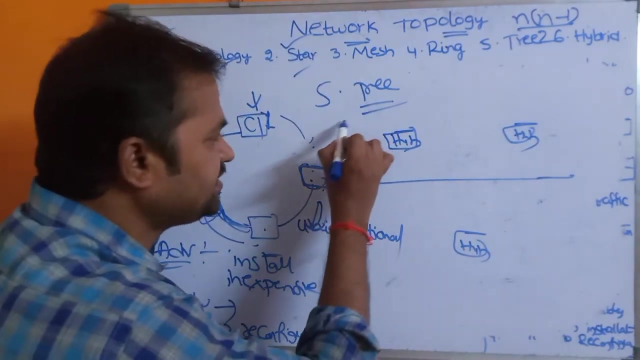 like this. So this is nothing but a long cable, just like the bus-toe policy. and then it is a combination of bus and star, So star means we can have hub. So this is one hub. This is the second hub, So this is the third hub. So this is nothing but star-toe policy, So we can have 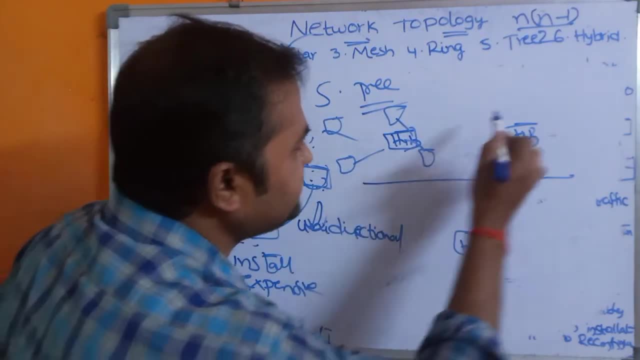 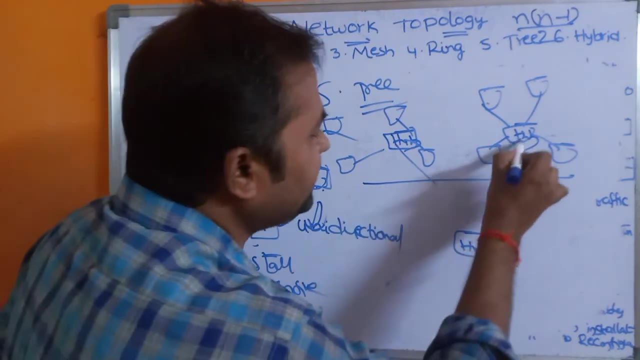 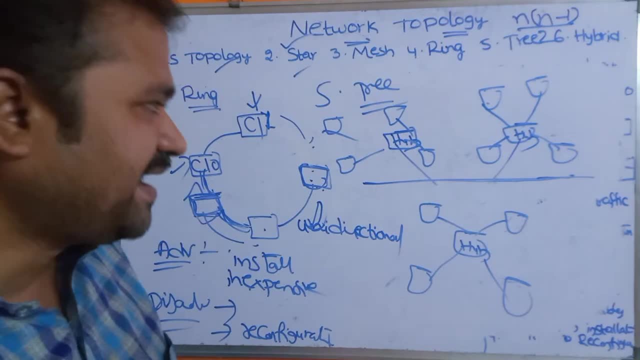 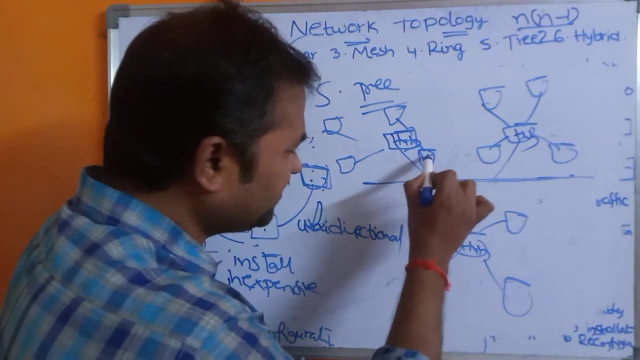 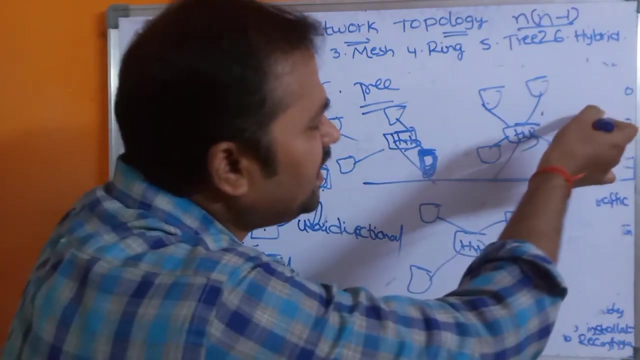 to the hub. So here the transmission will be done just like star-toe policy and bus-toe policy. but here the major advantage is: if one link fail, then there is no problem here. Why? Because this hub. if one link fails, then what we have is the remaining star-toe policies, The remaining 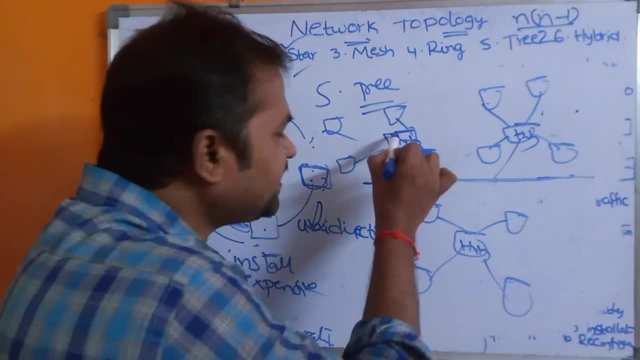 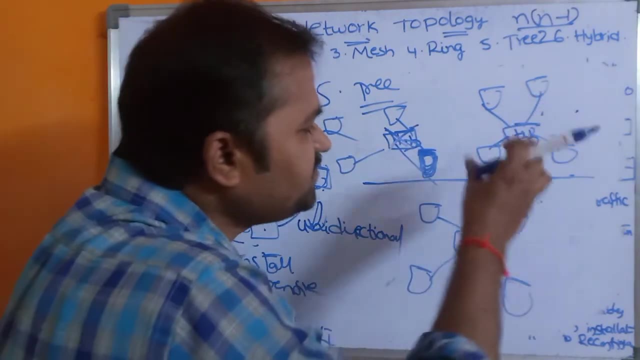 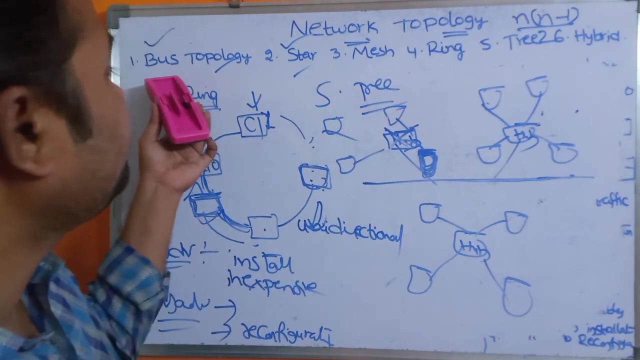 hubs will work. There is no problem here. Let us assume that this hub fails here. If this hub fails, then there is no problem. So we have two more hubs So we can transmit the data with the help of those two hubs. Coming to the advantages and disadvantages, three-toe policy has the advantages.